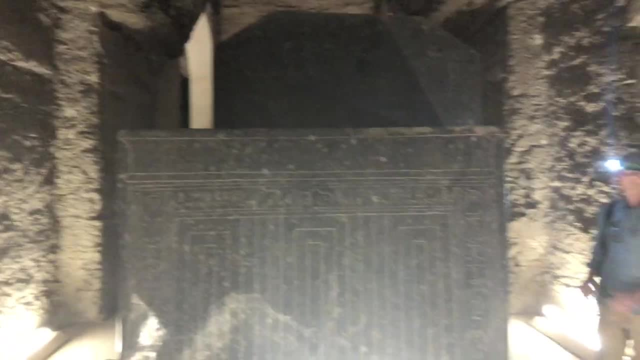 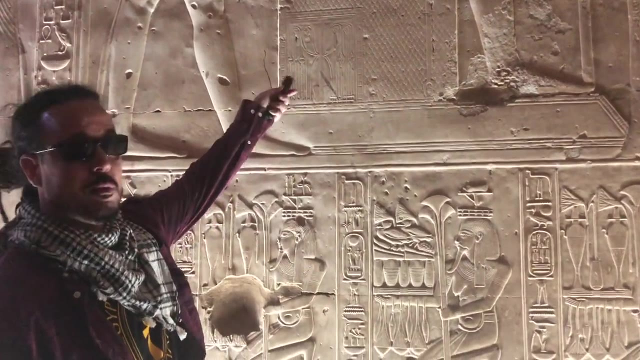 And once more, you'll be joining myself and author Chris Dunn for a hands-on, in-depth tour of Egypt, where, together, we'll study the evidence for lost technology and associated symbolism that's essential for ancient civilizations to exist. It's true, a hands-on expedition in Egypt. 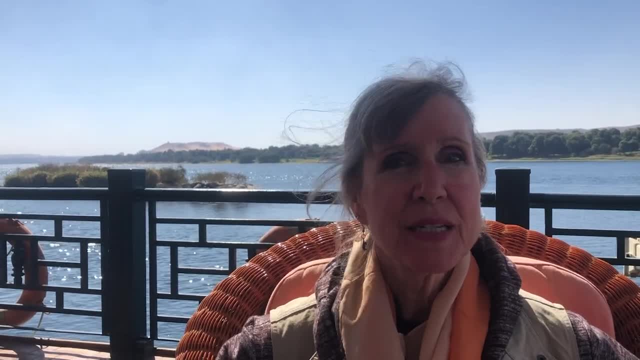 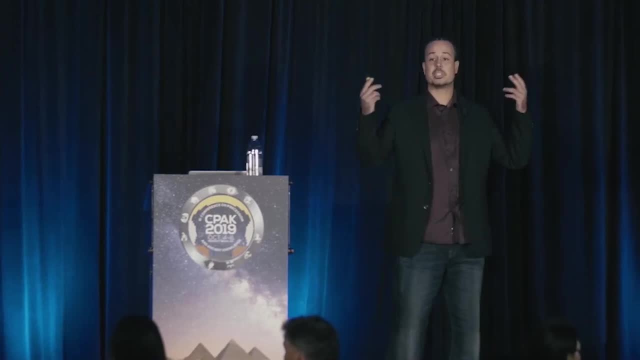 This tour to Egypt with NEXT and Adept Expeditions Has been a profound experience in my life. NEXT studied with John Anthony West, of course, but has decades of his own research, and he brings an independent and unique perspective to all of this. 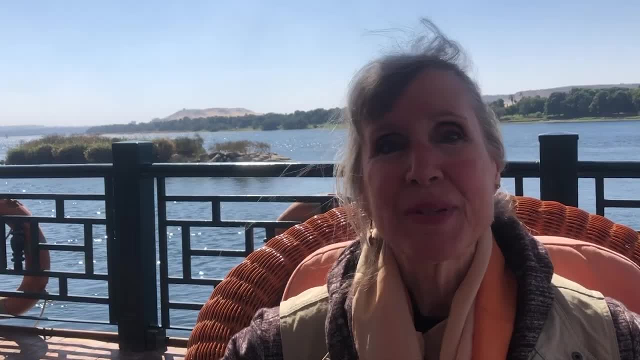 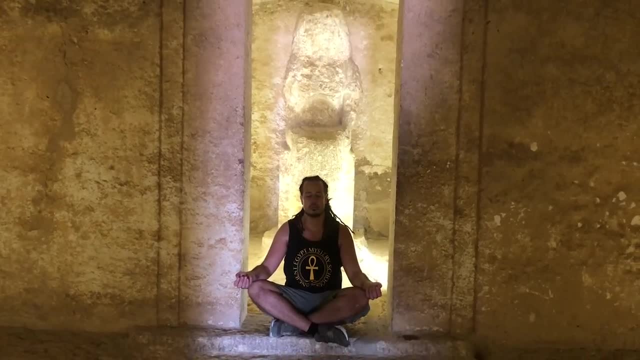